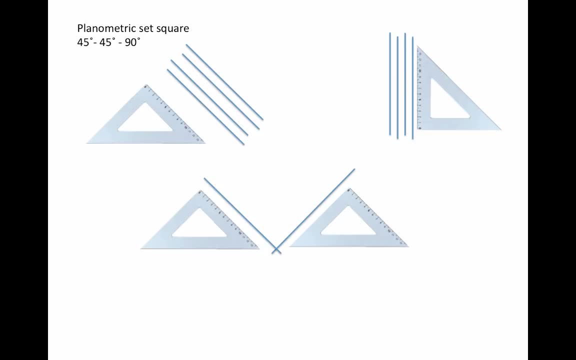 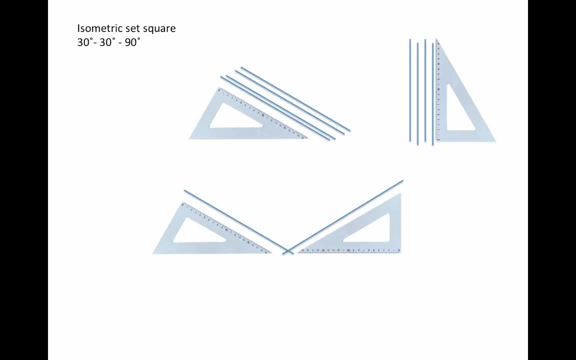 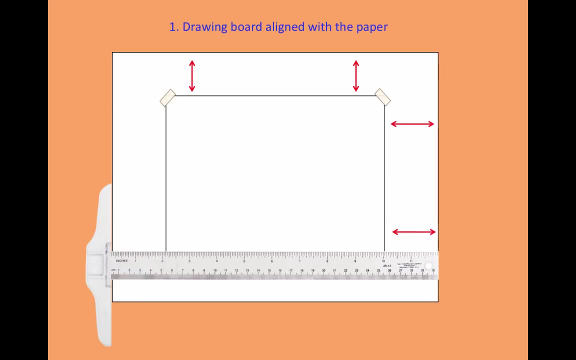 45 degree lines and 90 degree lines. Our isometric set square creates 30 by 30 by 90 lines. Of course, the actual set square itself has one side at 30, the other side at 60. We do not use the side that has 60.. Now to begin. we need to make sure that we understand. 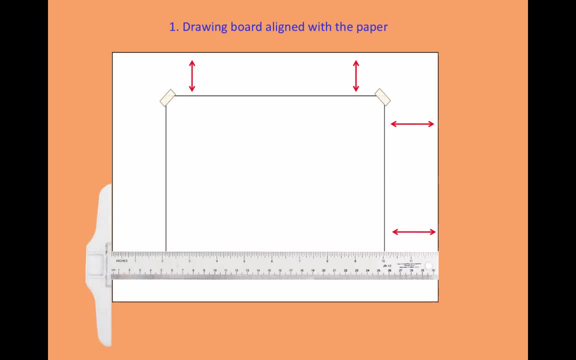